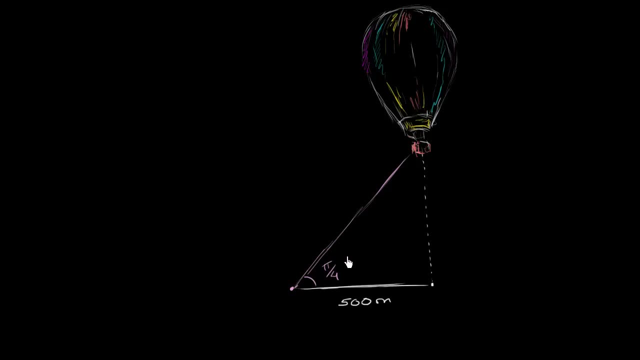 because when you take derivatives of trig functions, you assume that you're dealing with radians. So right over here this is pi over 4 radians And you also are able to measure the rate at which this angle is changing. So this is changing at 0.2 radians per minute. 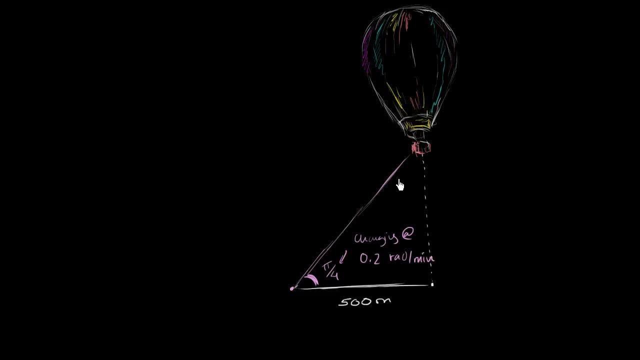 Now my question to you, or the question that you're trying to figure out as you watch this hot air balloon, is: how fast is it rising right now? How fast is it rising just as the angle between the horizontal and kind of the line? 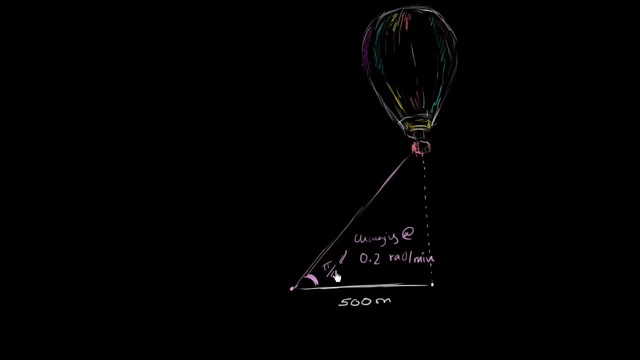 between you and the hot air balloon is pi over 4 radians, And that angle is changing at 0.2 radians per minute. So let's think about what we know and what we're trying to figure out. So we know a couple of things. 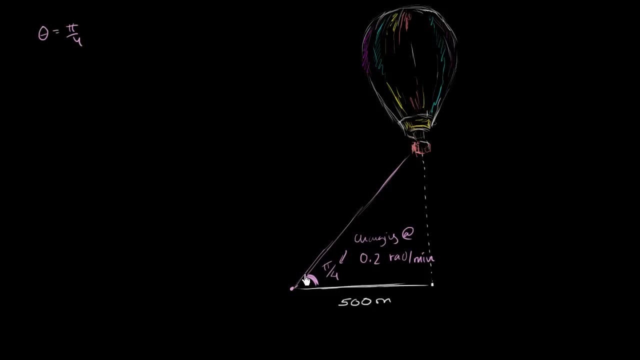 We know that theta is equal to pi over 4, if we call theta the angle right over here. So this is theta. We also know the rate at which theta is changing. We know d theta- let me do this in yellow. we know d theta. dt is equal to 0.2 radians per minute. 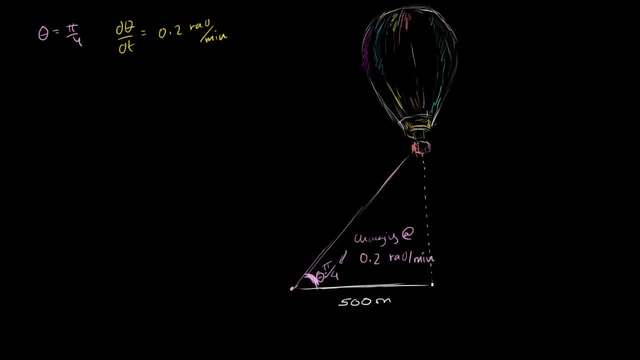 Now, what are we trying to figure out? Well, we're trying to figure out the rate at which the height of the balloon is changing. So, if you call this distance right over here, this distance right over here, h, what we want to figure out is dh, dh, dt. 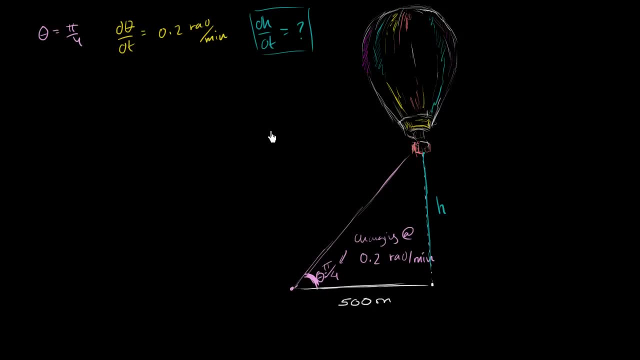 That's what we don't know. So what we'd want to come up with is a relationship between dh, dt, d, theta, dt and maybe theta if we need it, Or, another way to think about it, if we can come up with a relationship between h and theta. 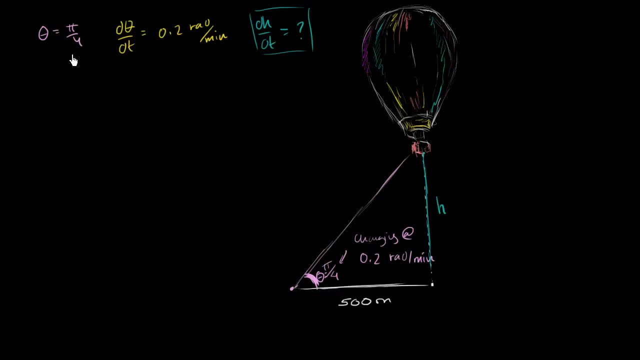 then we could take the derivative with respect to t and we'll probably get a relationship between all of this stuff. So what's the relationship between theta and h? Well, it's a little bit of trigonometry, We know. we're trying to figure out h. 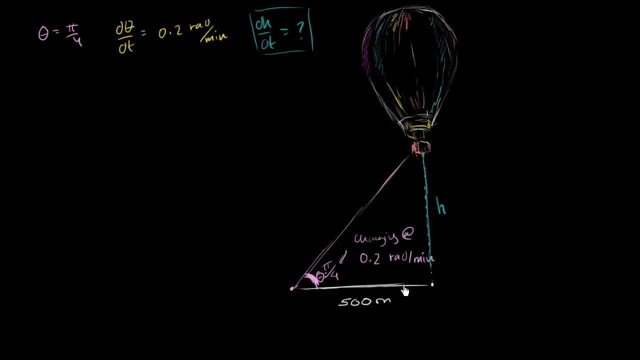 We know what this length is right over here. We know opposite over adjacent. that's the definition of tangent. So let's write that down. So we know that the tangent of theta is equal to the opposite side. The opposite side is equal to h over the adjacent side. 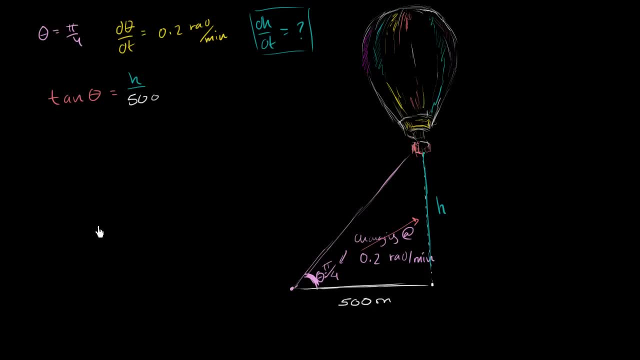 which we know is going to be a fixed 500.. So there you have a relationship between theta and h, And then to figure out a relationship between theta, d, theta and dh or d, theta, dt, the rate at which theta changes with respect to t. 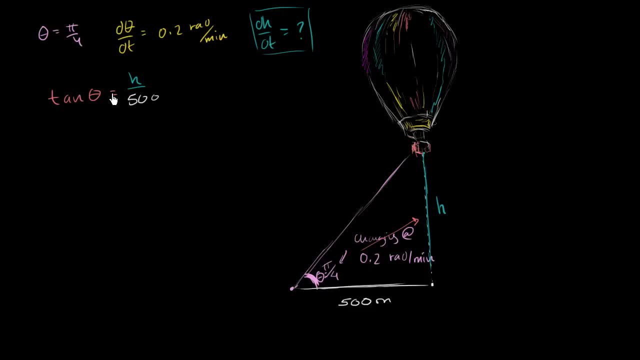 and the rate at which h changes with respect to t. we just have to take the derivative of this, of both sides of this with respect to t, implicitly. So let's do that And actually let me move over this h over 500 a little bit. 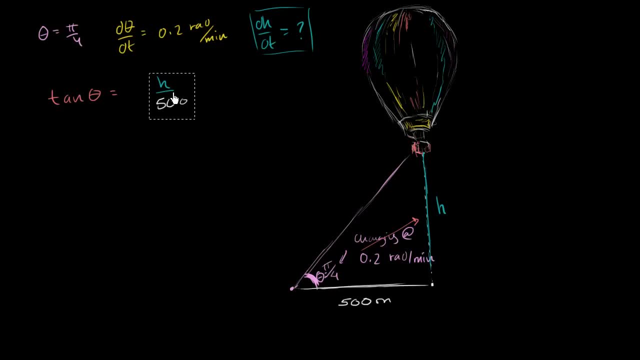 So let me move it over a little bit. so I have space to show the derivative operator, So let's write it like that. And now let's take the derivative with respect to t. So d, dt. we're going to take the derivative with respect. 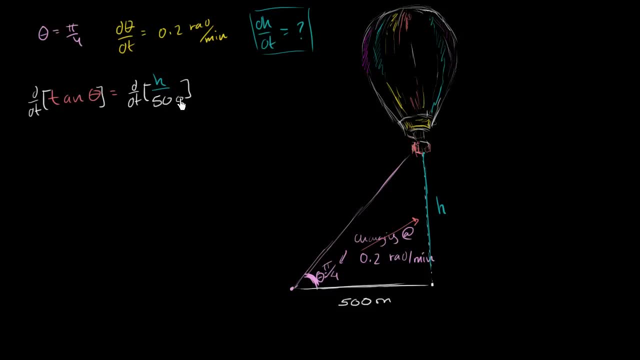 to t on the left. We're going to take the derivative with respect to t on the right. So what's the derivative with respect to t of tangent of theta? Well, we're just going to apply the chain rule here. It's going to be first the derivative. 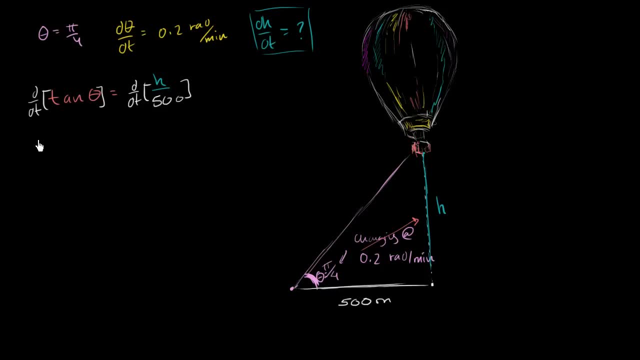 of the tangent of theta with respect to theta, which is just secant squared of theta times the derivative of theta with respect to t, Times d theta, dt. Once again, this is just the derivative of the tangent of something with respect to that something times the derivative of the something. 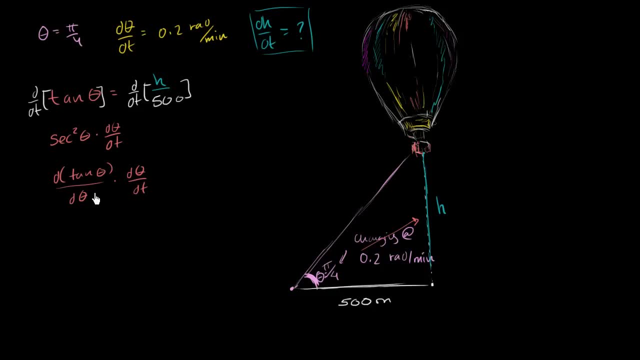 with respect to t. Derivative of tangent. theta with respect to theta times. the derivative of theta with respect to t gives us the derivative of tangent of theta with respect to t, which is what we'd want when we take d, when we use this type of a derivative operator. 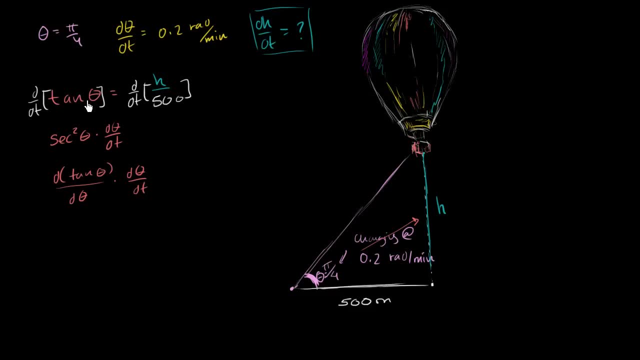 We're taking the derivative with respect to t, not just the derivative with respect to theta. Fair enough, so this is the left-hand side, and then the right-hand side becomes- well, it's just going to be one over 500 dh dt. 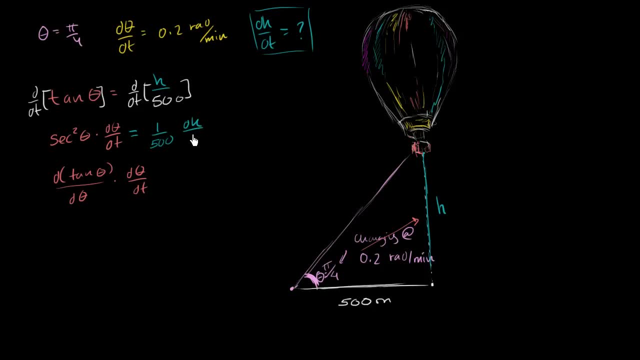 So one over 500 dh dt. We're literally saying it's just one over 500 times the derivative of h with respect to t. But now we have our relationship. We have the relationship that we actually care about. We have a relationship between the rate. 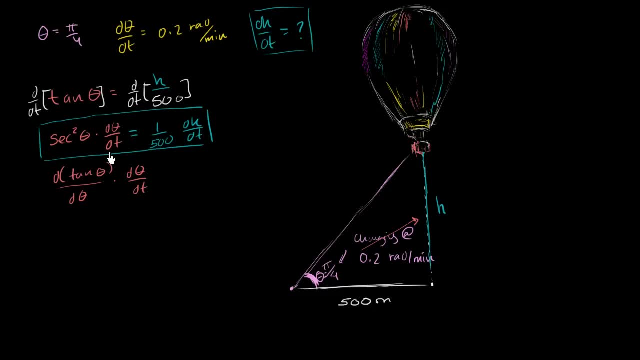 at which the height is changing with respect to time and the rate at which the angle is changing with respect to time and our angle at any moment. So we can just take these values up here, throw it in here and then solve for the unknown. 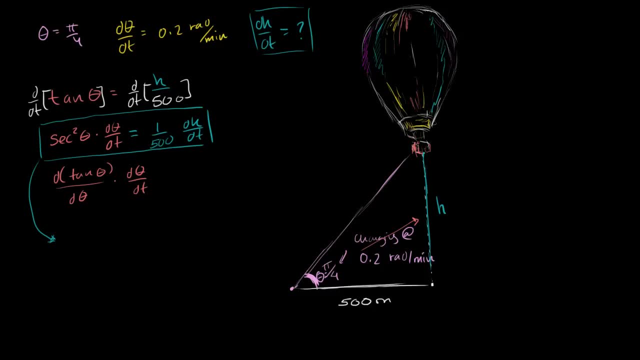 So let's do that, Let's do that right over here, So we get secant squared of theta. So we get secant squared Right now our theta is pi over 4.. Secant squared of pi over 4.. Let me write those colors in to show you. 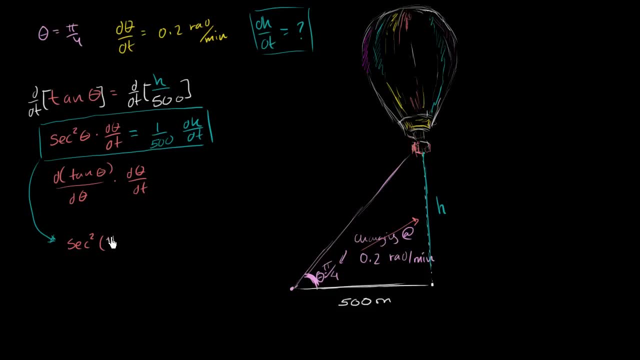 that I'm putting these values in Secant squared of pi over 4 times d theta dt. Well, that is just 0.2. So times 0.2. And then this is going to be equal to one over 500.. 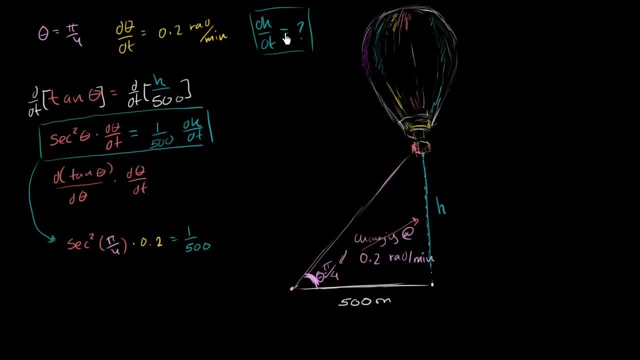 And we want to make sure, since this is in radians per minute, we're going to get meters per, And this is meters right Over here. We're going to get meters per minute right over here. We just want to make sure we know what our units are doing. 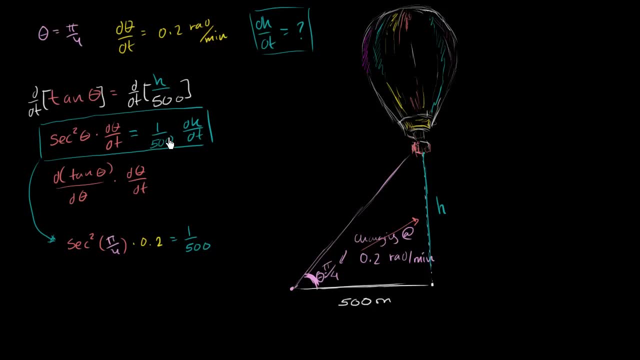 I haven't written the units here to save some space, But we get 1 over 500 times dh dt. So if we want to solve for dh dt, you can multiply both sides by 500. And you get the rate at which our height is changing. 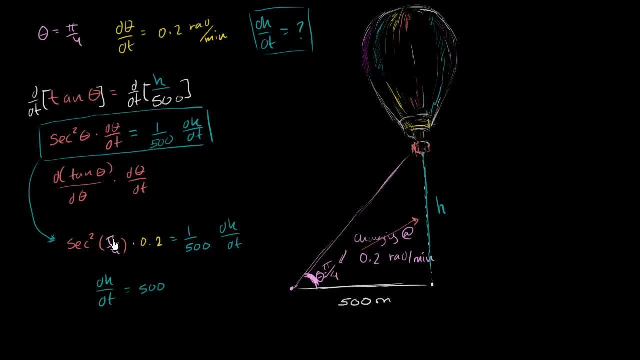 is equal to 500 times. let's see secant squared of pi over 4.. That is 1 over cosine, squared of pi over 4.. Let me write this over: Cosine of pi over 4 is square root of 2 over 2.. 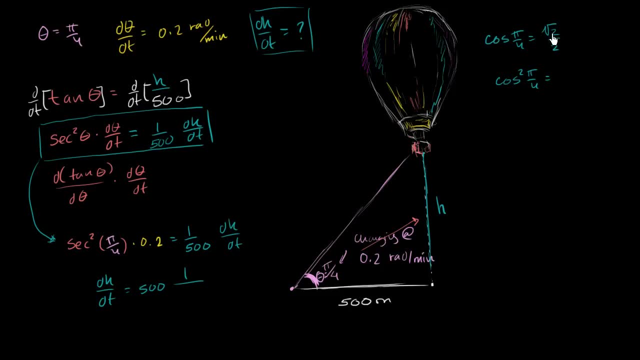 Cosine, squared of pi over 4 is going to be equal to 2 over 2 over 4, which is equal to 1 1⁄2.. And so secant squared of pi over 4 is just 1 over that. 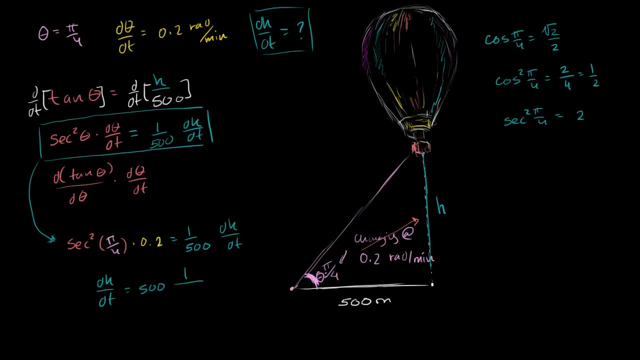 is equal to 2.. So this is going to be equal to- let me rewrite this instead of: So the secant squared of pi over 4.. Let me erase this right over here. Secant squared of pi over 4, all of this business.